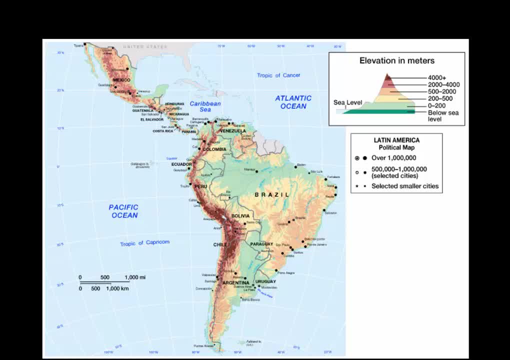 But it extends from Mexico all the way down to southern Chile. here, And here's a map of it. You notice it doesn't include this country right here: Belize, the Caribbean and these three countries here: Guyana, French Guyana, which belongs to France, and Suriname. 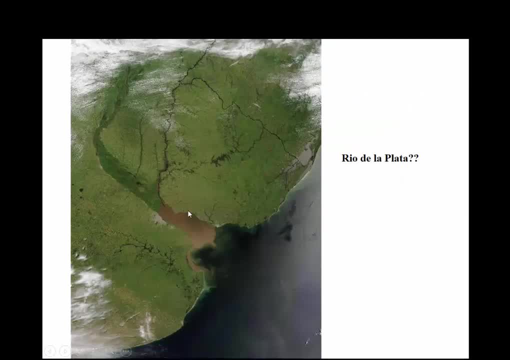 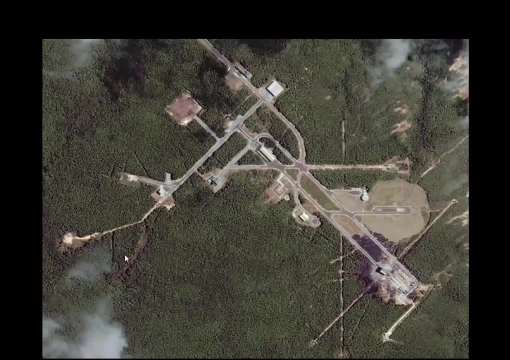 You can see the Rio de la Plata which separates Uruguay and Argentina. Here's some satellite imagery because a lot of times Europe has their launching facilities in- I believe it's French Guyana, and there's some places in Brazil because it's closer to the equator. 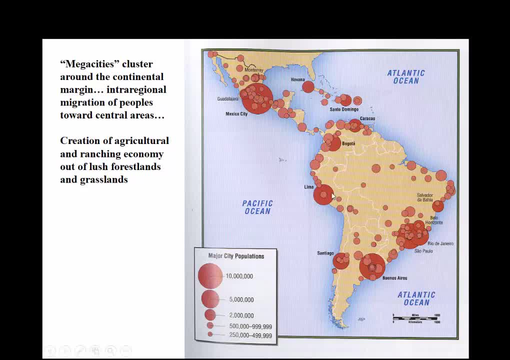 And you can see the megacities that go around the periphery of South America. and then, of course, you can see Mexico City. here You can see places like Lima, Bogota, of course, Mexico City, Buenos Aires, Sao Paulo, Rio, up and down the coast here. 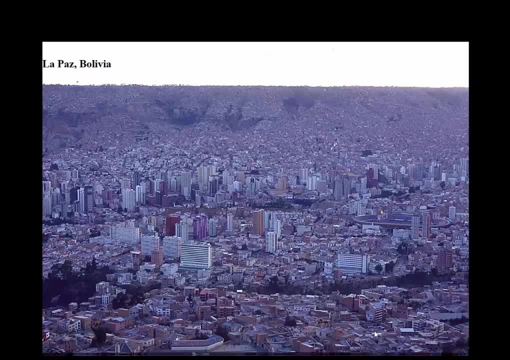 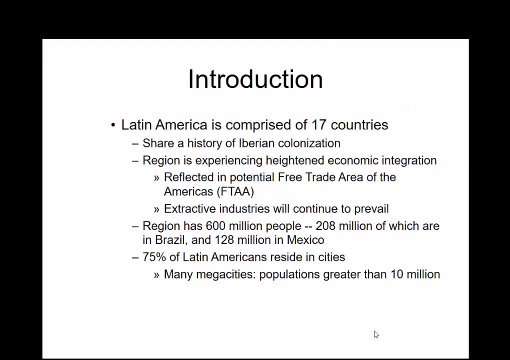 So we'll talk about and refer to that term later- megacities. You can see La Paz, Bolivia, which is one of the two landlocked countries in South America. But Latin America is composed of about 17 countries. It shares a history of Iberian colonization. 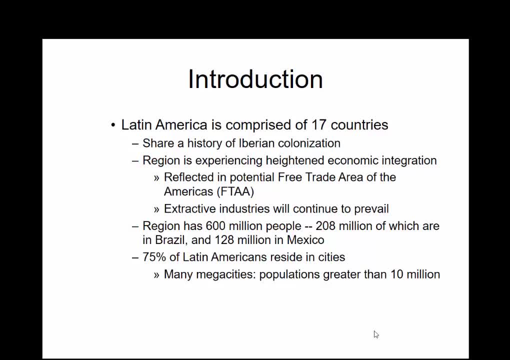 Iberian refers to the countries of Portugal and Spain. It contains about 600 million people, so a little bit less than 10% of the world's population. There's more than 200 million in Brazil. There's about 128 million in Mexico. 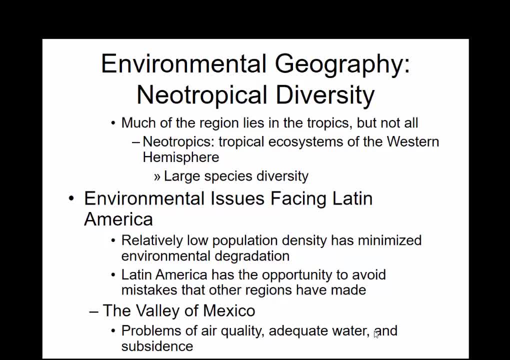 When we talk about the neotropical diversity, one of the big issues- environmental issues especially facing Latin America- is that issues, especially in Mexico, issues of air quality, water quality and subsistence- Actually the actual country or the actual city is sinking because of the weight of Mexico City in that valley. 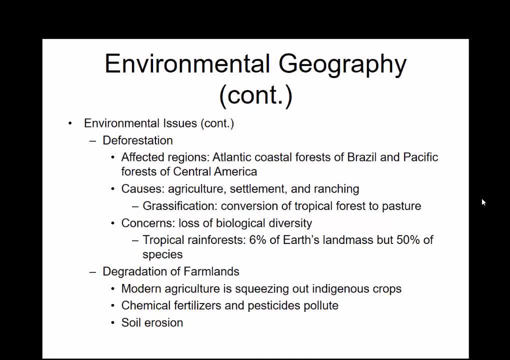 Other issues we deal with are deforestation, especially in places such as the Amazon, and the loss of what we call biodiversity- Six percent of the Earth's land mass. In terms of tropical rainforests, we have 50% of the world's species. 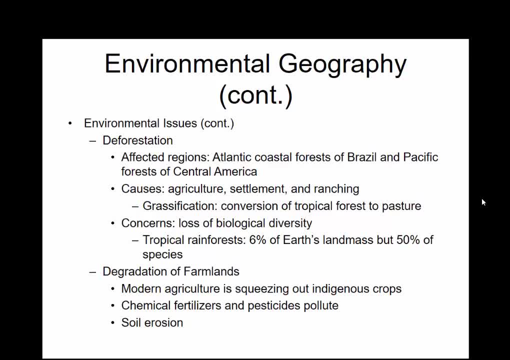 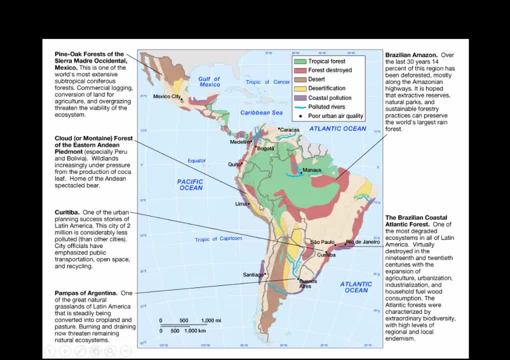 That turns into things like chemical fertilizer, soil erosion, some of the things we alluded to before. You can see the Amazon rainforest here In the middle of Amazon. it does extend briefly into Colombia, but when we talk about the Amazon, we're mainly talking about Brazil. 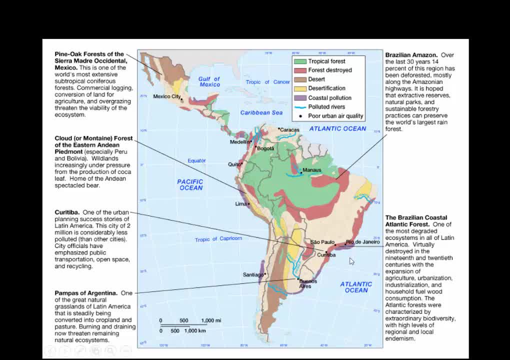 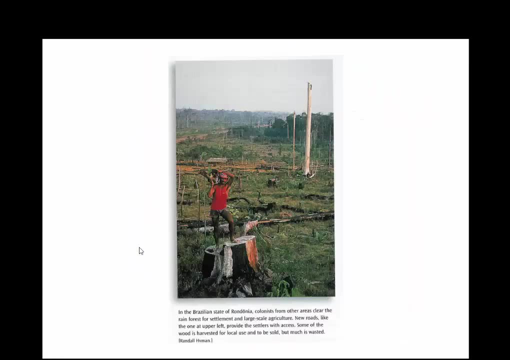 These are some of the environmental issues. We have coastal pollution- Remember the 2016 Rio Olympics- Coastal pollution with swimming events or open water- swimming, rather and sailing, was a concern- And then some of these polluted rivers. You can see this is the Brazilian state where they're clearing. 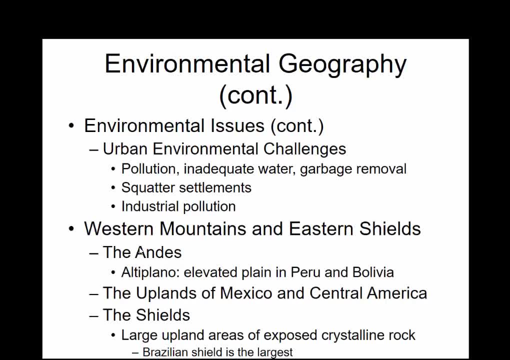 This is along the Amazon, And then other things like environmental challenges- and we'll refer to those later- And then some of the physical regions that we do have. We have the Western Mountains, we've got the Andes, which run pretty much up the spine of South America. 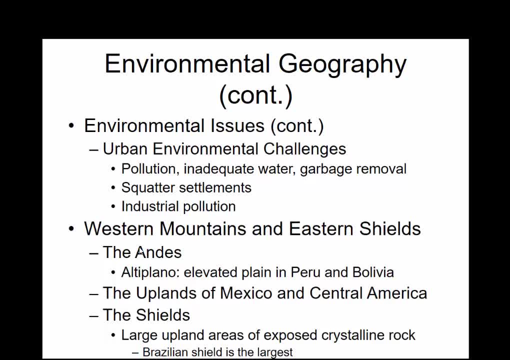 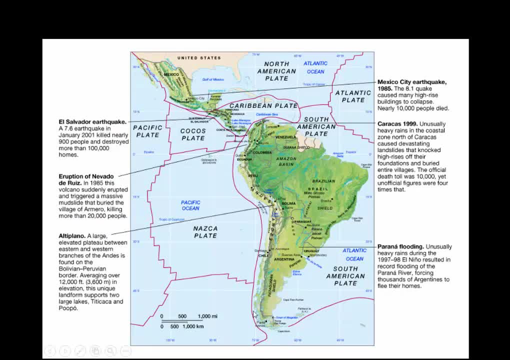 And then we've got the Shields, large upland areas of exposed crystal and rock, And then you can see a map here of South America. So we've got the separation, the boundary between the South American plate and the Nazca plate, where it meets up here with the Caribbean plate. 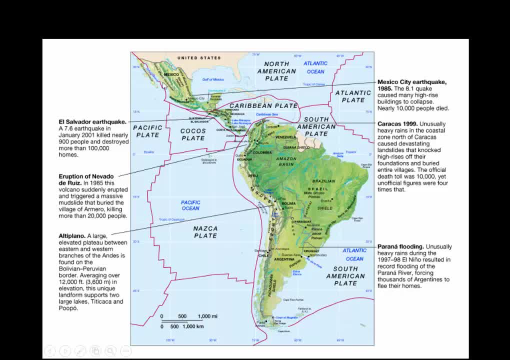 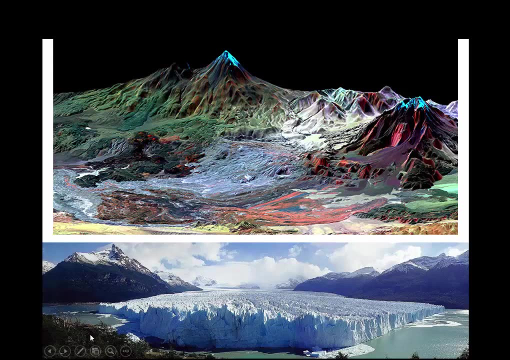 So we've got a lot of volcanic and tectonic activity in Mexico, Chile, Peru, Colombia, Not as much over there, It's not as much over in Brazil, And you can see down in the south, here, the far south, we have glaciers. 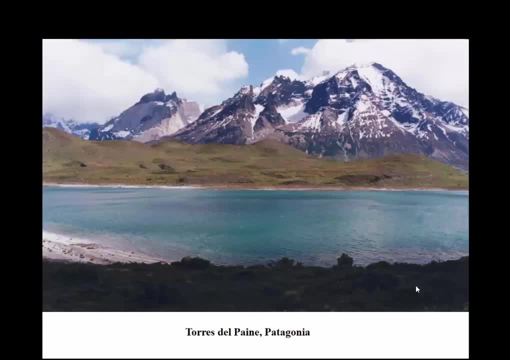 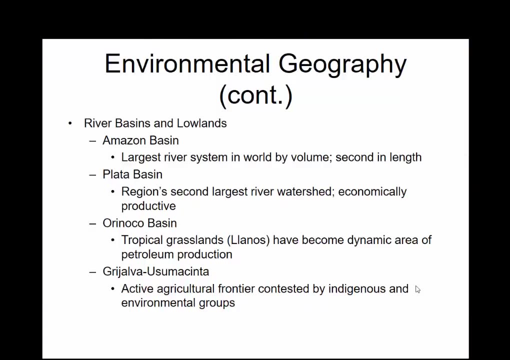 And what we call Tierra del Fuego. This is in Patagonia. This is a sparsely populated area in southern Argentina. So we have places like the Orinoco in the northern part of South America, the Palo Alto, The Plata Basin, Rio de la Plata and the Amazon. 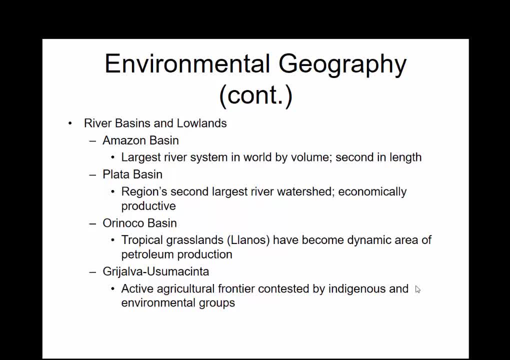 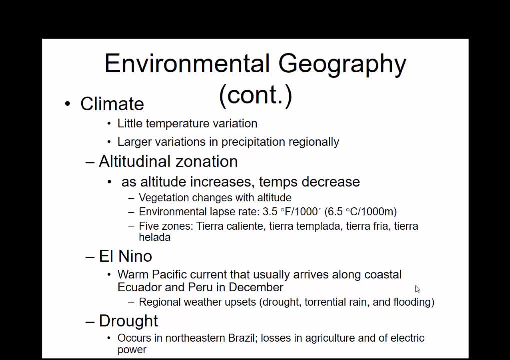 It's the largest river system by volume but the second in length- the Nile- And you can see some of the environmental, geography and the physical issues that they deal with: Drought, El Nino, altitudinal zonation, because we do have stark temperature changes. 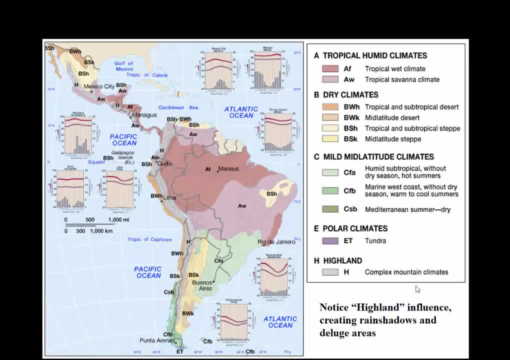 So it has a number of different zones as you move further and further up And you can see some of the climate regimes here. A lot of these are going to be your A's. you know tropical wet. We don't even know what tropical wet is. 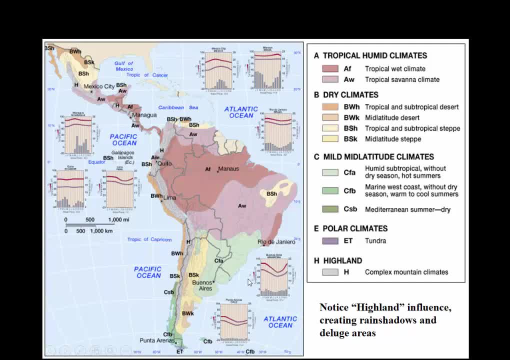 And you can get down to any of the D's, like we do see in Canada and we'll look at in Russia. But we've got our highlands that run right along the spine right here And we do have some highlands here up in Mexico City where mountains get really high. 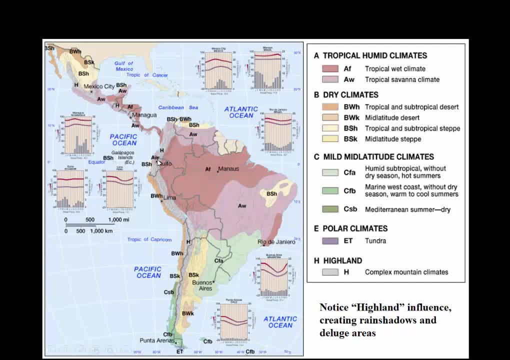 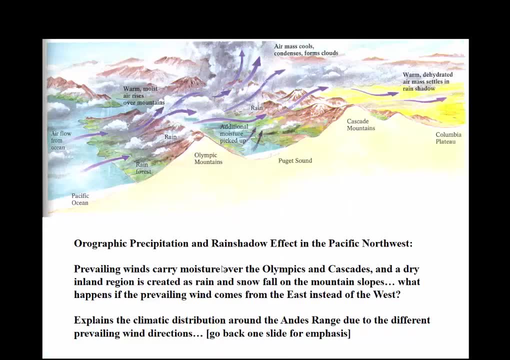 And these are fairly complex, but we can see, you know, our desert-like conditions over here, And we'll refer to those at a much smaller scale, or a larger scale rather, Speaking of which we have something called orographic precision. 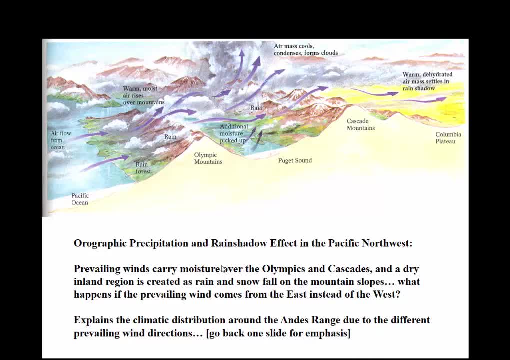 When we look at precipitation and something called relative humidity, it's specific humidity divided by the saturation humidity. And as rain moves up the saturation, the ability for water to hold air decreases. So at some point in time it gets to 100% relative humidity. gets to 100% relative humidity. 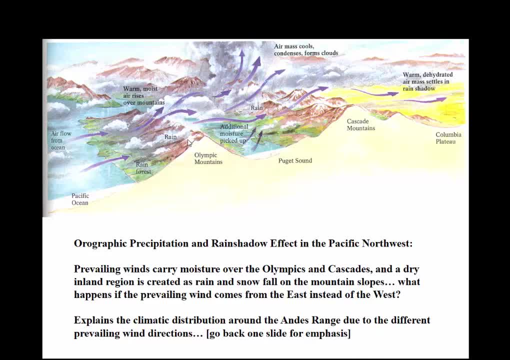 and eventually needs to precipitate, whether or not it's going to precipitate or not, So it's going to precipitate. So it's going to precipitate, whether or not it's going to precipitate, whether or not it's going to precipitate. 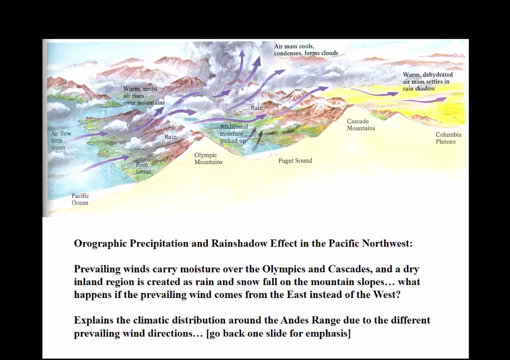 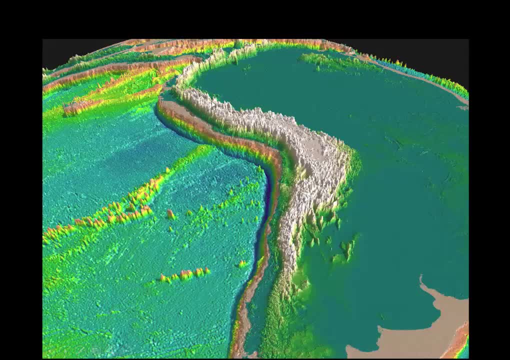 whether in the form of sleet, snow, rain or whatever here. So we have these rain shadows. This is an example here in the Olympic Mountains as we look to the Columbia Plateau. But this you can see the example here with the Andes Mountains right here. 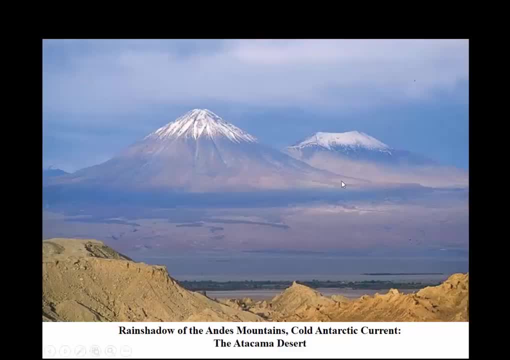 and then, stuck inside of the Andes, we have some of these deserts which receive very little precipitation. This is the rain shadow. so on the far side of the Andes Mountains, this cold Antarctic current which typically doesn't hold a lot of water to. 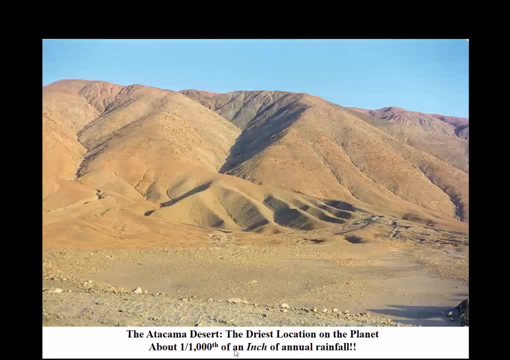 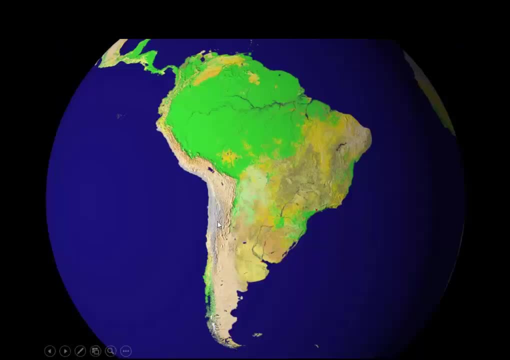 begin with, we have the Atacama Desert and this is one of the driest places on the surface of the earth and you can see- we're kind of looking at this region right here, but you can see the rain shadow down here in Patagonia. okay, as a 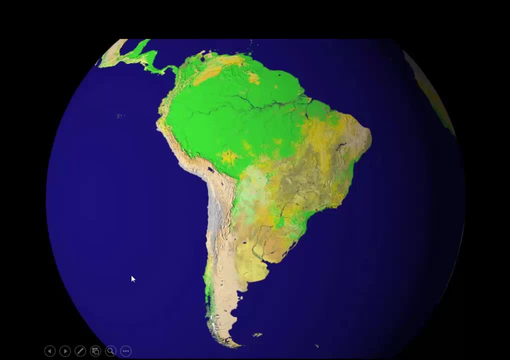 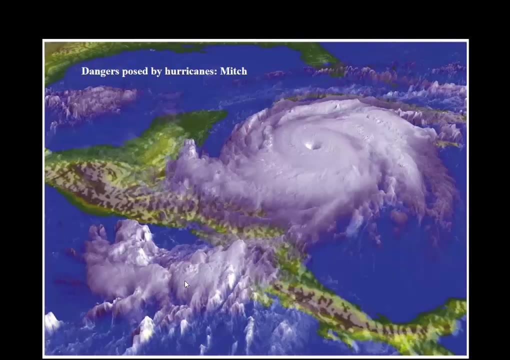 result of this rain shadow effect from water and circulation patterns coming from the Southern Pacific Ocean, Antarctic, we can see dangers posed by Hurricane Mitch in Central America. they don't get too much into South America. here this is Hurricane Mitch and I think this was in the 90s. in 2012, I went on a 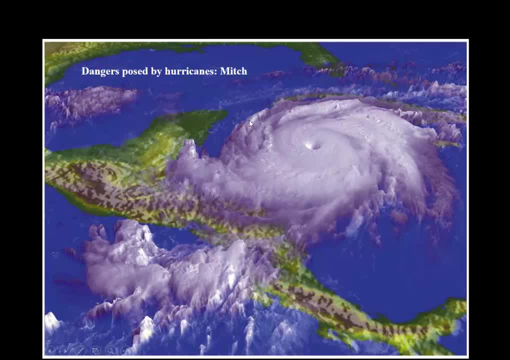 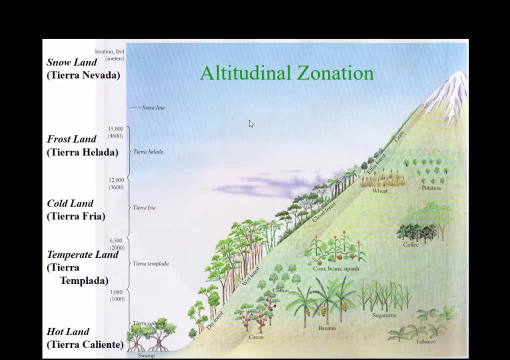 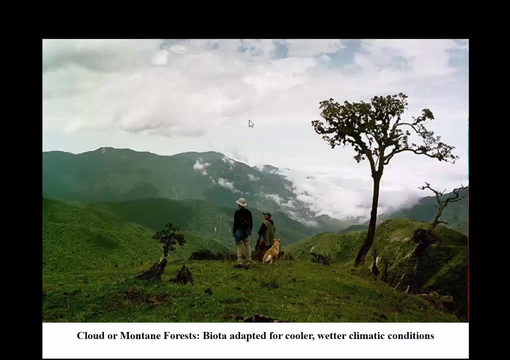 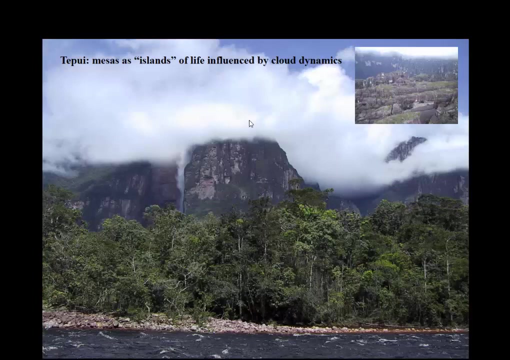 cruise through Mexico, in Central America, and we were diverted because one of the hurricanes there- and like I was talking about before, this is the altitude nozomation cloud, or montane for us biota, adopted by cooler, wetter climate conditions and the same relative latitude longitude, but change slightly due to elevation. these 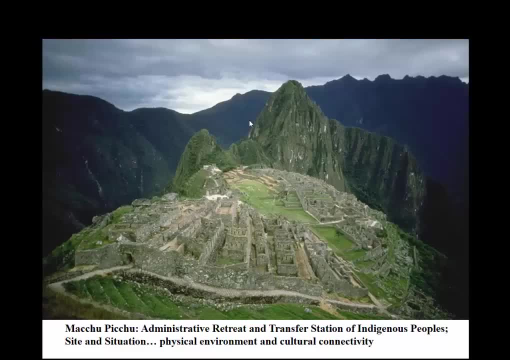 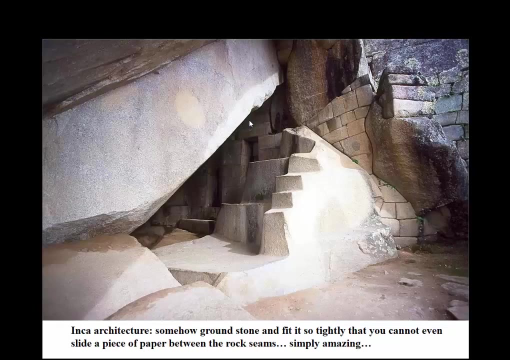 are maces of islands influenced by cloud dynamics. most pronounced is these: Machu Picchu. this is the administrative retreat and transfer station of the indigenous people and you can see the relationship between the physical environment and this cultural connectivity here. and this the main map here. this is the main map. if we turn on the screen here right now, we're 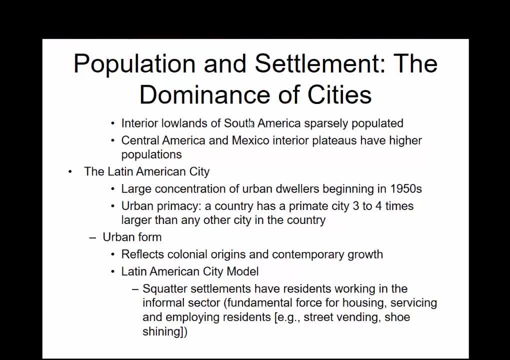 When we look at more cultural patterns and settlement patterns, we've got the Latin American city. It's a large concentration. It's typically what we call urban primacy or primate cities. It's basically a city that has three to four times larger than any other city in the country. 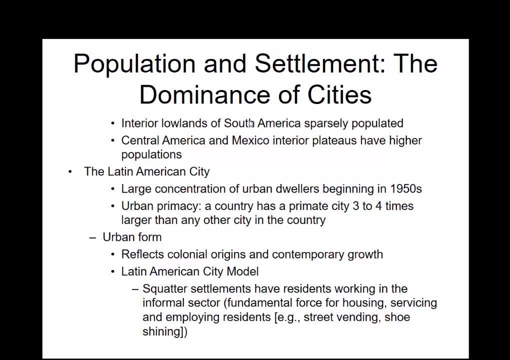 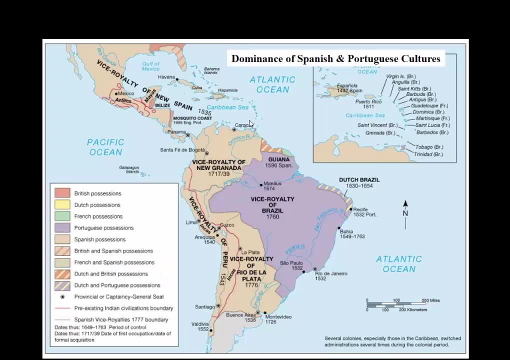 A lot of times, when we say Peru, we think Lima. When we think of Colombia, we say Bogota. When we say Chile, we say Santiago. We don't really know too many other cities because they're so much larger than those. We have the Spanish dominance in Portuguese cultures. 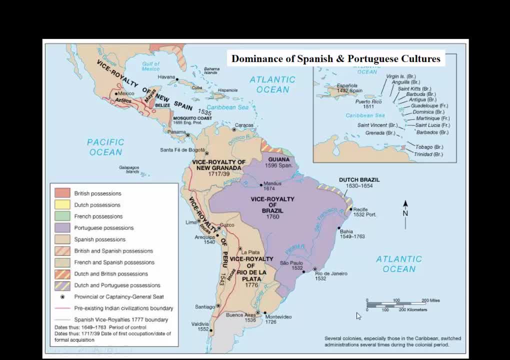 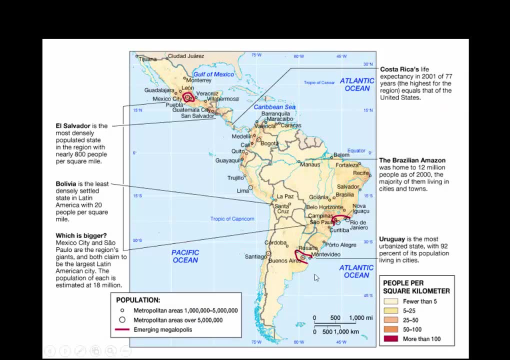 We can see the history of this. Talk about this Iberian colonization. You can see a dot density map of where people are. We've got Montevideo, Sao Paulo, Rio de Janeiro around the periphery. here It's for a variety of reasons. 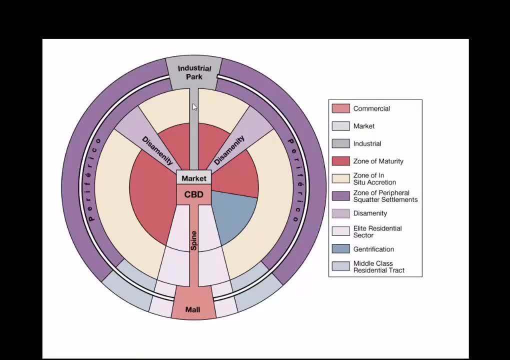 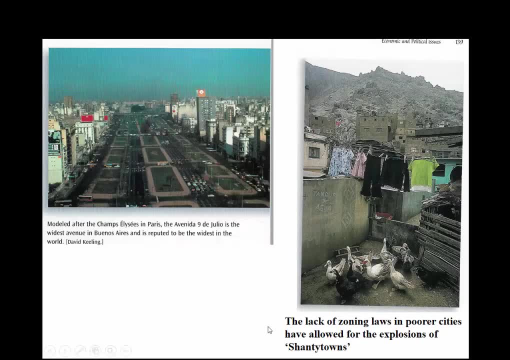 And, of course, Mexico City. You can see an example of your typical South American city, but these change a lot. Lock of zoning laws in poorer cities. You saw this at the Olympics with Rio de Janeiro- And then we see planned cities. 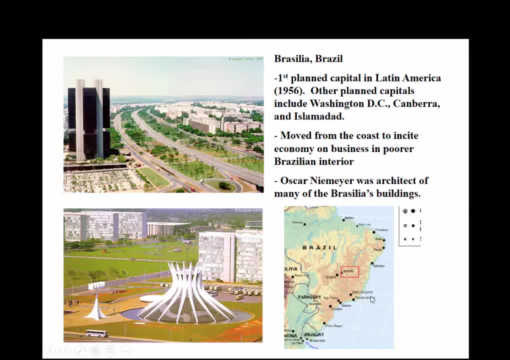 Such as Brasilia, who's moved inland to stimulate the economy, inland from Rio de Janeiro and Buenos Aires or Sao Paulo, I'm sorry- moved inland to serve as a capital. So this is a planned capital. It was the first planned capital in Latin America in 1956. 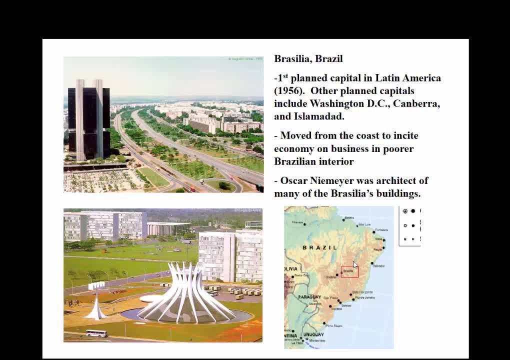 There's other planned capitals. Believe it or not, Washington DC was a planned capital. It was in the middle of the country at the time. Canberra is an example. New Zealand- I'm sorry, Australia- is an example of a planned capital. 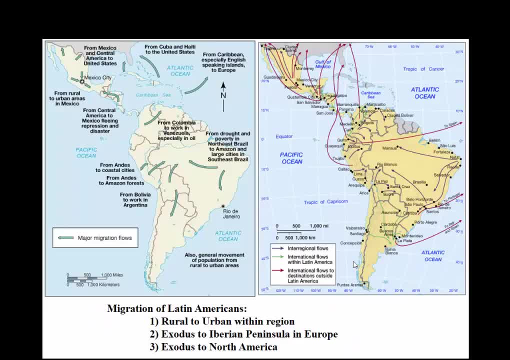 And Abuja, Nigeria, is an example of a planned capital. So you can see the migration of Latin America, this rural to urban within the region, And then you see this exodus to the Iberian Peninsula in Europe or an exodus to North America. 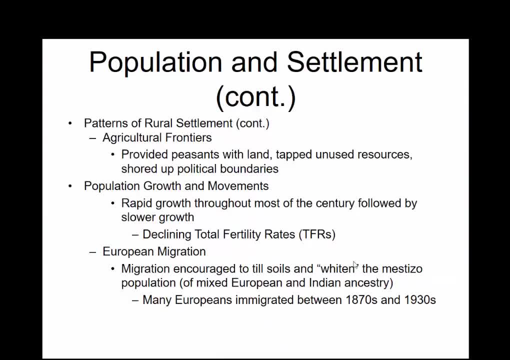 So you can see a lot of this inter- and intra-regional migration. We've got rapid population growth and a lot of that is due to we do have a lot of population growth. We do have declining fertility rates but more importantly, or what contributes to that- a lot more. 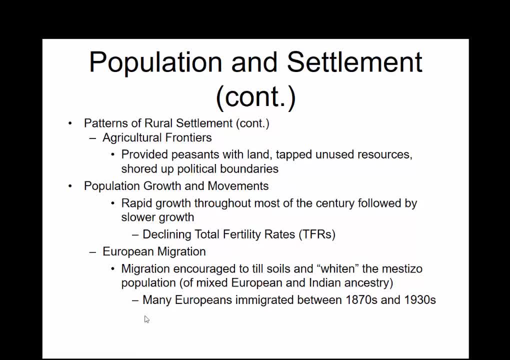 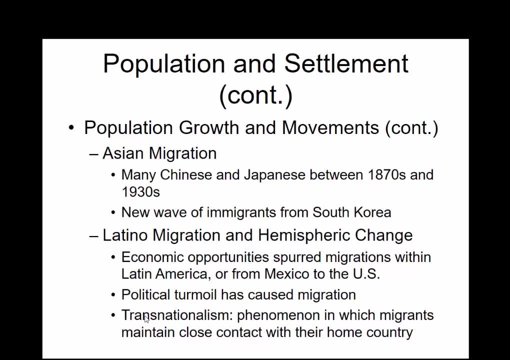 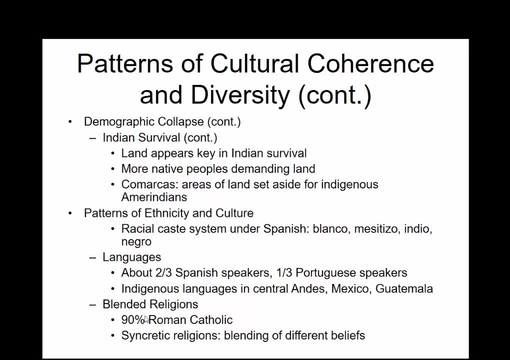 is the decrease in crude death rates. We've had a lot of Chinese and Japanese between the 1870s and 1930s, so you see, that's very big. And then we talk about languages, about two-thirds Spanish speakers, one-third Portuguese speakers. 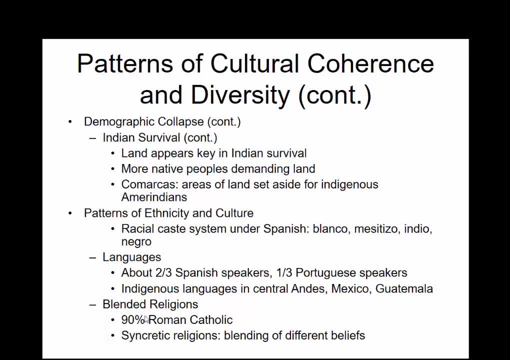 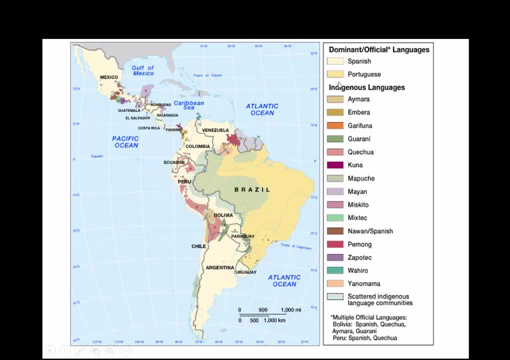 And we've got indigenous languages in your Central Andes, Mexico, Guatemala, and it's mainly Roman Catholic. It's based on the predominance of from Portugal and Spain And you can see some of the dominant languages here. you know, obviously, Spanish and Portuguese. 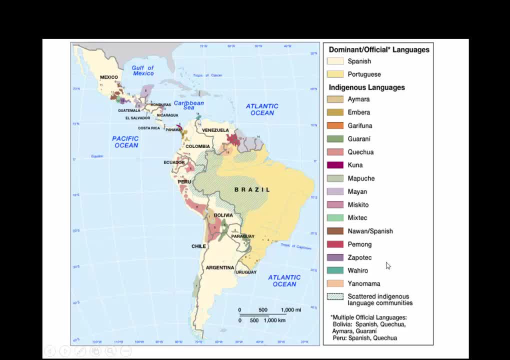 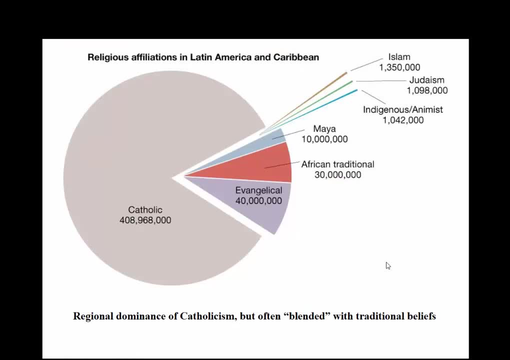 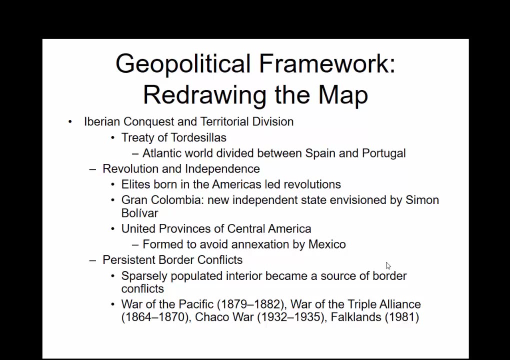 but like we have here in these maps, we do have some indigenous or local languages, And this is just a map here or this is just the graph of language, sorry, religion, Like we said before the Treaty of Tordesillas, basically the Atlantic world. 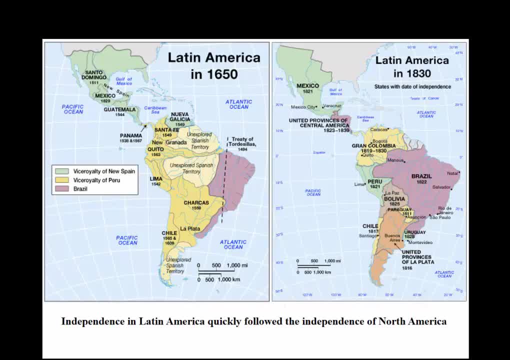 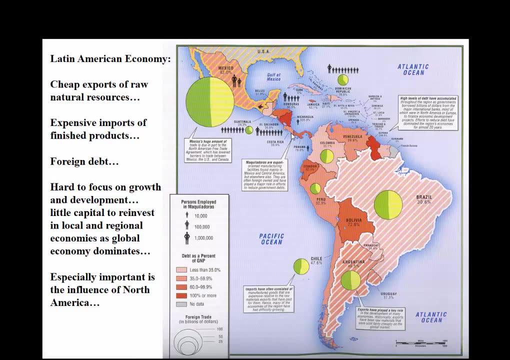 it was divided between Spain and Portugal And I'll kind of look at a map of it here so you can see the Portuguese influence here. and then pretty much the rest was Spain moving up into North America into the 1800s. This is the Latin American economy. you know the cheap exports of raw natural resources. 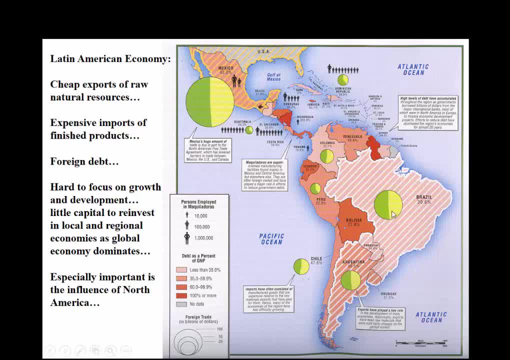 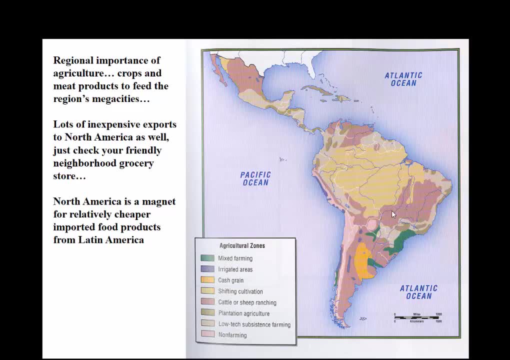 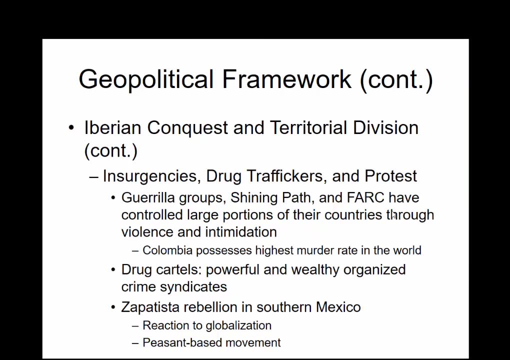 okay in this Amazon area right here. And then the regional importance of agriculture. Other things about geopolitics- we've had insurgencies. drug traffickers- We heard about those in the 80s with the country of Colombia- drug cartels-